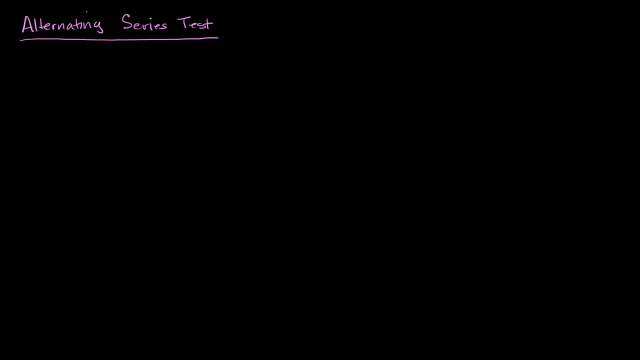 Let's now expose ourselves to another test of convergence and that's the alternating series test, And I'll explain the alternating series test and I'll apply it to an actual series while I do it, to make the explanation of the alternating series test a little bit more concrete. 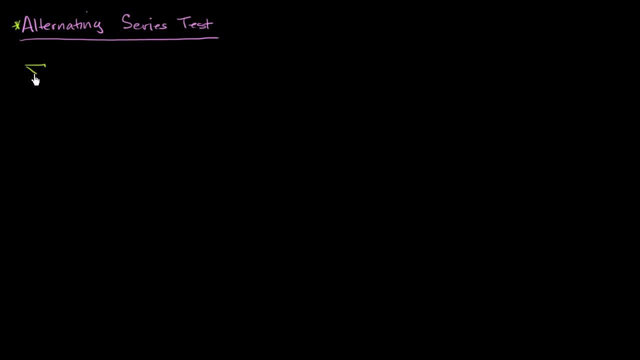 So let's say that I have some series, some infinite series. Let's say it goes from n equals k to infinity of a sub n and let's say I can write it as or I can rewrite a sub n. So let's say a sub n I can write. 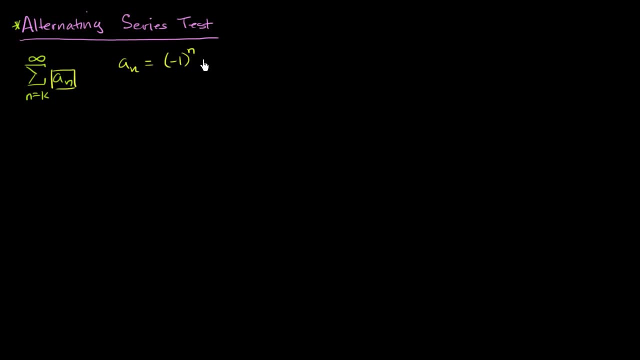 so a sub n is equal to negative one to the n times b sub n. or a sub n is equal to negative one to the n plus one times b sub n, where b sub n is greater than or equal to zero. for all the n's we care about. 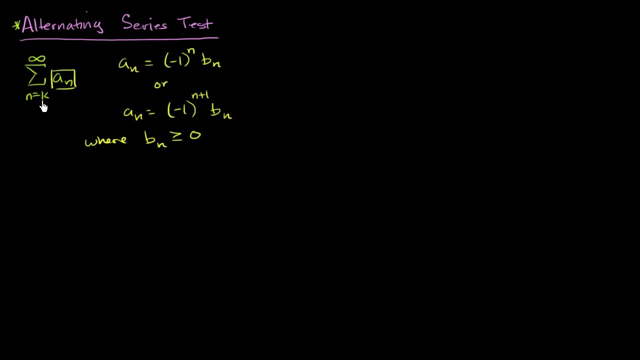 So, for all of the n's, we care about all of these integer n's greater than or equal to k. So if all of these things, if all of these things are true, and we know two more things, and we know number one. 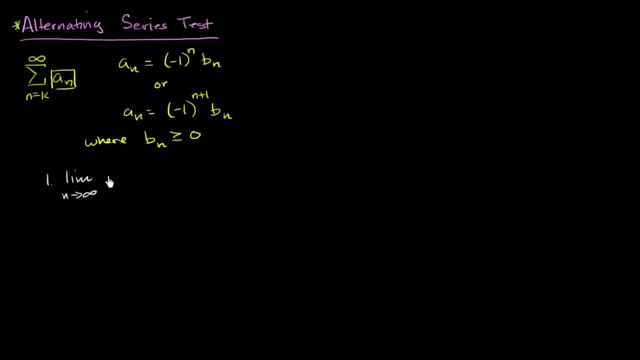 the limit. as n approaches, infinity of b sub n is equal to zero and number two, b sub n is a decreasing sequence. decreasing sequence, then that lets us know that the original infinite series, the original infinite series, is going to converge. So this might seem a little bit abstract right now. 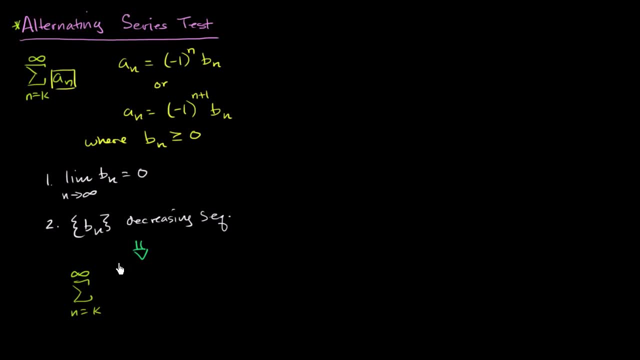 Let's actually show, let's use this with an actual series to make it a little bit more, a little bit more concrete. So let's say that I had the series. let's say I had the series. let's say I had the series from n equals one to infinity. 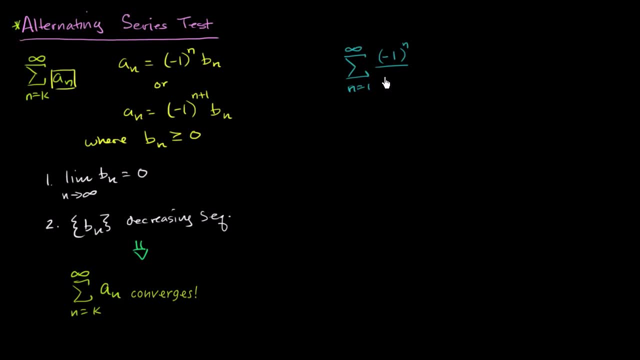 of negative one to the n over n, And we could write it out just to make this series a little bit more concrete: When n is equal to one, this is going to be negative one to the one power. actually, let's just make this: 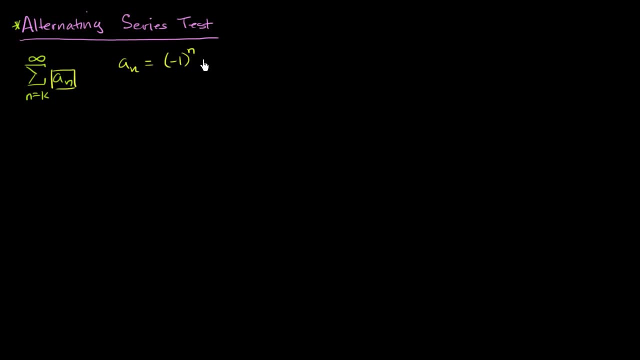 so a sub n is equal to negative one to the n times b sub n. or a sub n is equal to negative one to the n plus one times b sub n, where b sub n is greater than or equal to zero. for all the n's we care about. 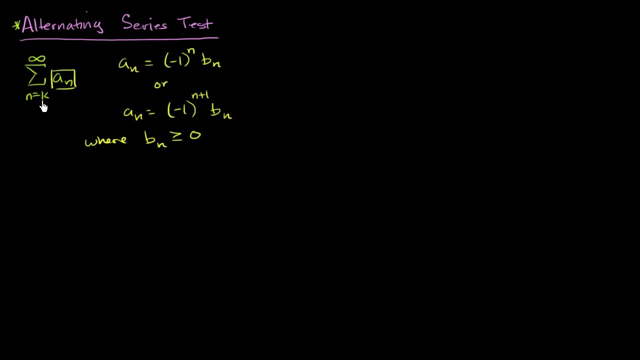 So, for all of the n's, we care about all of these integer n's greater than or equal to k. So if all of these things, if all of these things are true, and we know two more things, and we know number one. 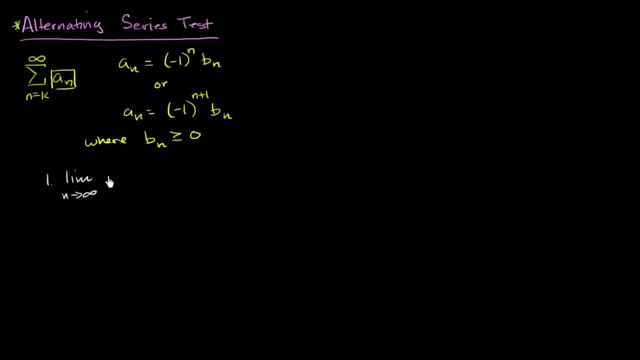 the limit. as n approaches, infinity of b sub n is equal to zero and number two, b sub n is a decreasing sequence. decreasing sequence, then that lets us know that the original infinite series, the original infinite series, is going to converge. So this might seem a little bit abstract right now. 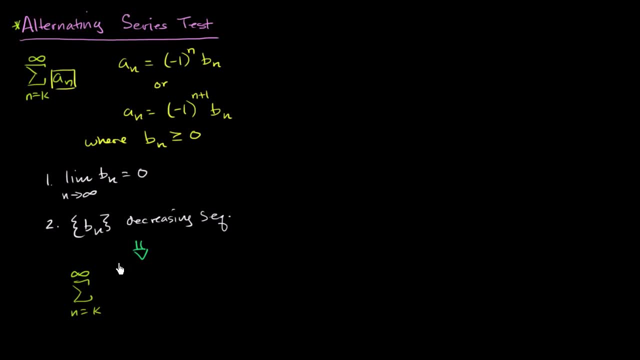 Let's actually show, let's use this with an actual series to make it a little bit more, a little bit more concrete. So let's say that I had the series. let's say I had the series. let's say I had the series from n equals one to infinity. 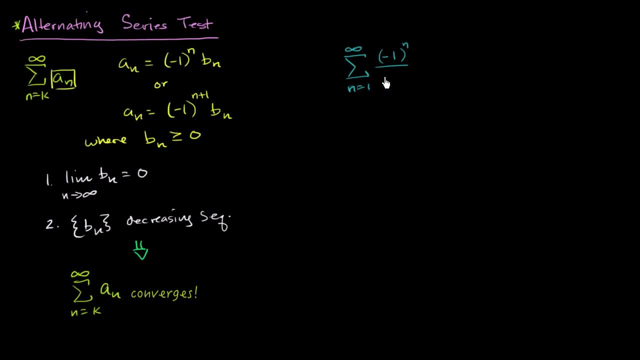 of negative one to the n over n, And we could write it out just to make this series a little bit more concrete: When n is equal to one, this is going to be negative one to the one power. actually, let's just make this: 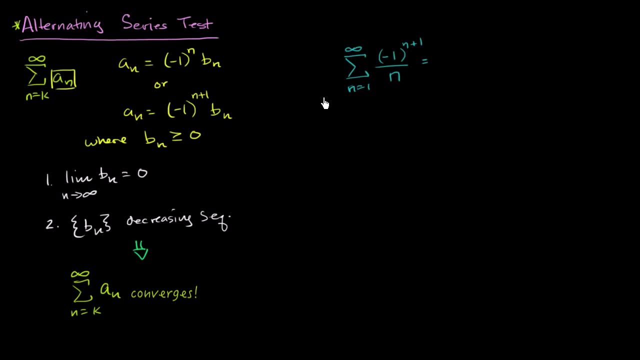 a little bit. let's make this a little bit more interesting. Let's make this negative one to the n plus one. So when n is equal to one, this is going to be negative one squared over one which is going to be one. 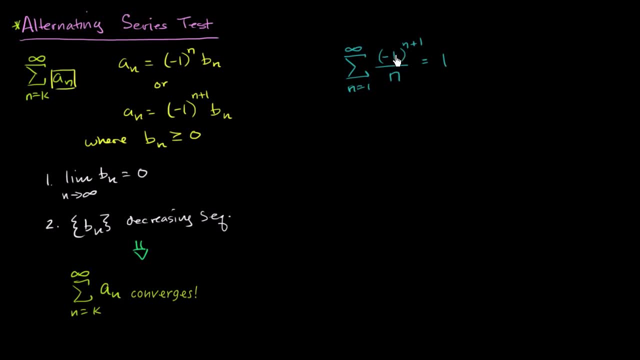 and then when n is two, it's going to be negative one to the third power, which is going to be negative one half. so it's minus one half plus one, third minus one fourth plus minus. and it just keeps going on and on and on forever. 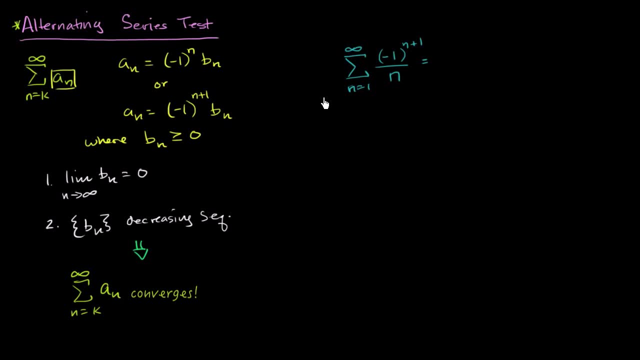 a little bit. let's make this a little bit more interesting. Let's make this negative one to the n plus one. So when n is equal to one, this is going to be negative one squared over one which is going to be one. 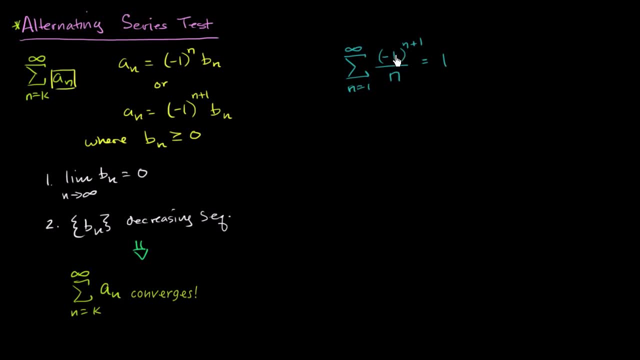 and then when n is two, it's going to be negative one to the third power, which is going to be negative one half. so it's minus one half plus one, third minus one fourth plus minus. and it just keeps going on and on and on forever. 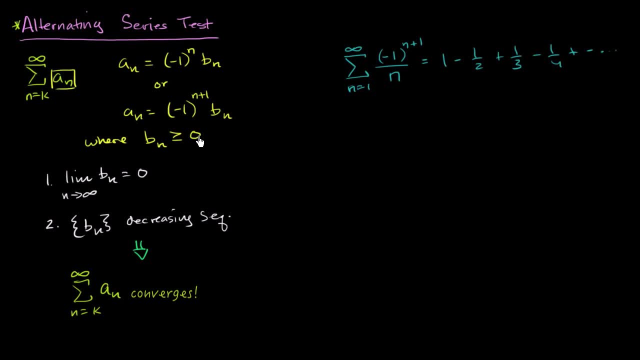 Now can we rewrite this, a sub n like this: Well, sure, the negative one to the n plus one is actually explicitly called out. We can rewrite. we can rewrite our a sub n, so let me do that. So a sub n which is equal to negative one. 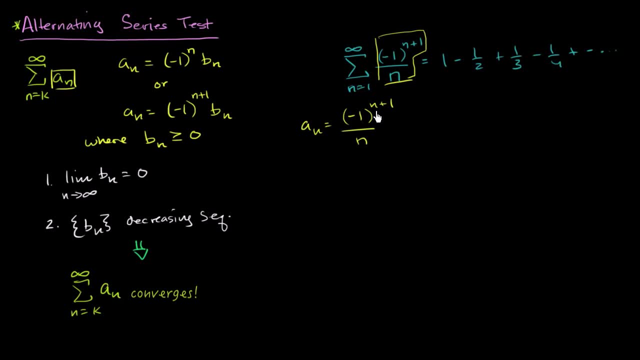 to the n plus one over n. This is clearly the same thing as negative one to the n plus one times one over n, which is which we can then say: this thing right over here could be our b sub n. So this right over here is our b sub n. 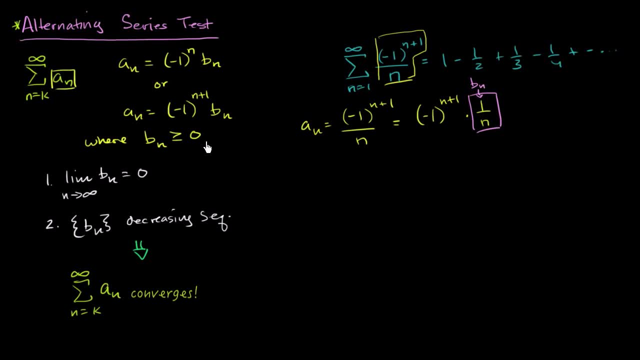 And we can verify that our b sub n is going to be greater than or equal to zero for all the n's we care about Subtitles by the Amaraorg community. So our b sub n is equal to one over n. Now, clearly, this is going to be greater than or equal to zero. 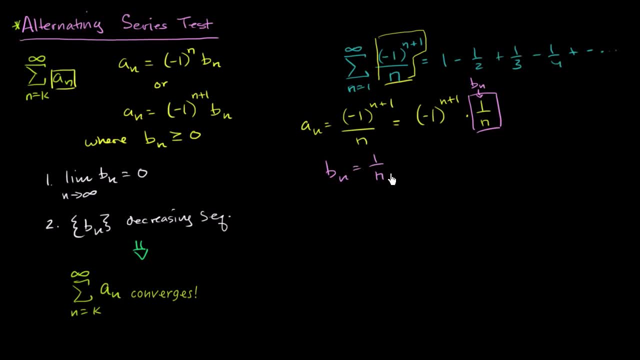 for any positive n. Now what's the limit of b sub n as n approaches infinity? The limit of, let me just write one over n. one over n as n approaches infinity is going to be equal to zero. So we satisfy the first constraint. 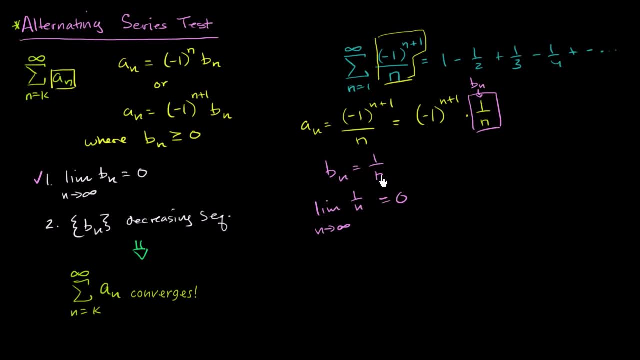 And then this is clearly a decreasing sequence. As n increases, the denominators are going to increase, and with a larger denominator you're going to have a lower value. So we can also say: one over n is a decreasing sequence for the n's that we care about. 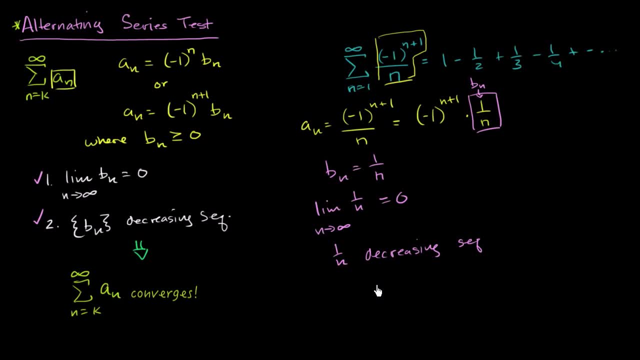 So this is satisfied as well, And so, based on that, this thing right over here is always greater than or equal to zero. The limit as one over n, or as our b sub n as n approaches infinity, is going to be zero. 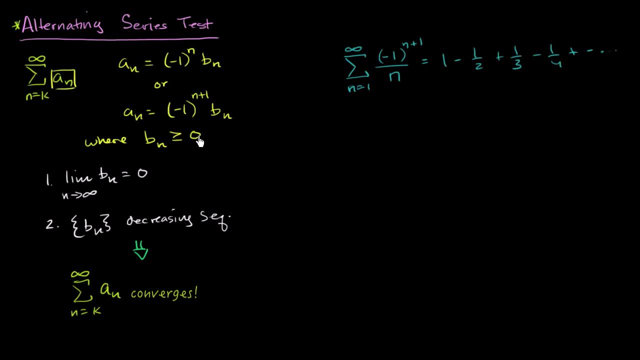 Now can we rewrite this, a sub n like this: Well, sure, the negative one to the n plus one is actually explicitly called out. We can rewrite. we can rewrite our a sub n, so let me do that. So a sub n which is equal to negative one. 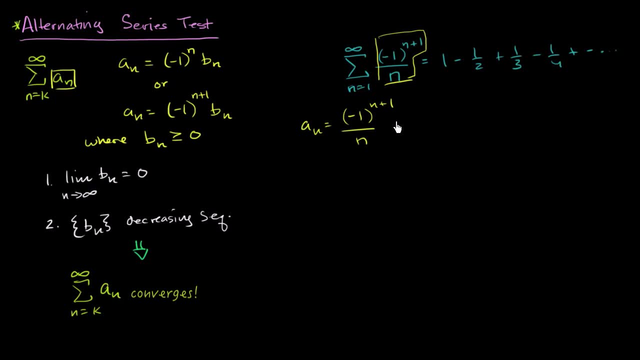 to the n plus one over n. this is clearly the same thing as negative one to the n plus one times one over n, which is which we can then say: this thing right over here could be our b sub n. So this right over here is our b sub n. 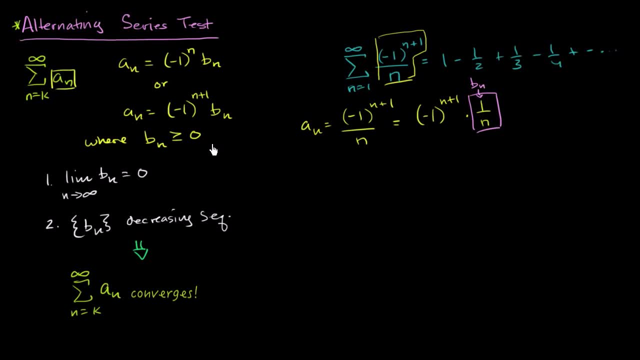 And we can verify that our b sub n is going to be greater than or equal to zero for all the n's we care about. So our b sub n is equal to one over n. Now, clearly, this is going to be greater than or equal to zero. 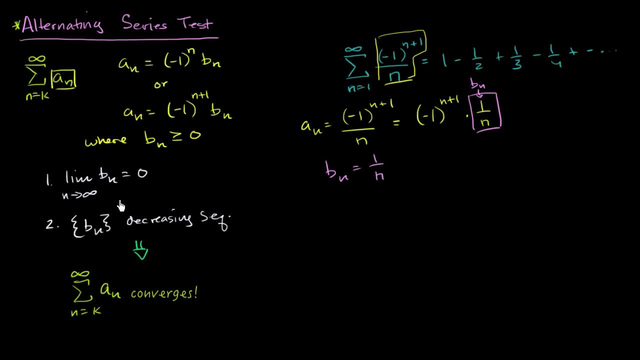 for any, for any positive n. Now, what's the limit as b sub n? what's the limit of b sub n as n approaches infinity? The limit of, let me just write one over n. one over n as n approaches infinity is going to be equal to zero. so we satisfy the first constraint. 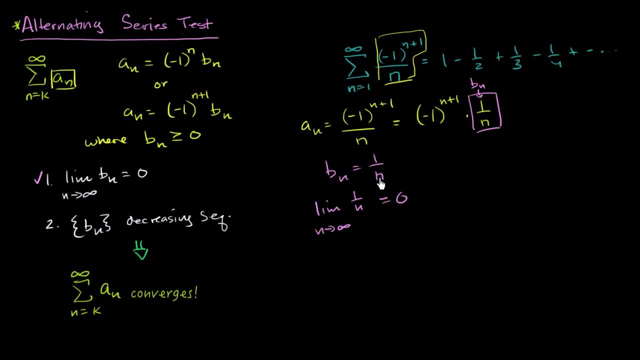 And then this is clearly a decreasing sequence as n. as n increases, the denominators are going to increase, and with a larger denominator you're going to have a lower value. So we can also say: one over n is a decreasing, decreasing sequence for the n's that we care about. 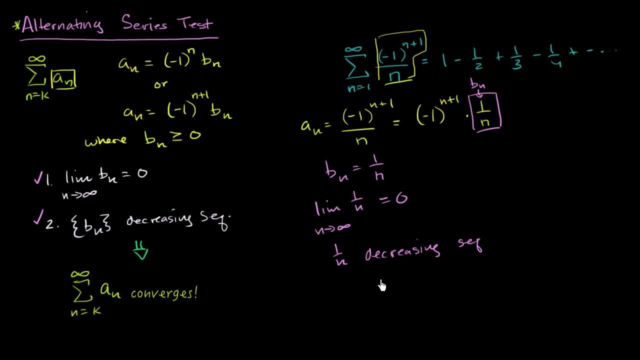 So this is this satisfies, this is satisfied as well, And so, based on that, this thing, this thing is always, this thing right over here is always greater than or equal to zero. The limit as one over n or as our b sub n. 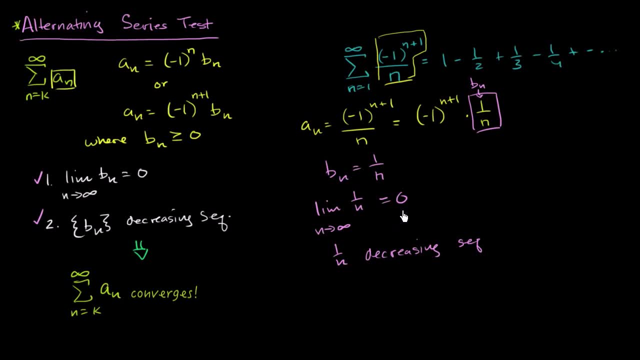 as n approaches, infinity is going to be zero. It's a decreasing sequence. therefore we can say that our original series actually converges. So n equals one to infinity of negative, one to the n, plus one over n. And that's kind of interesting because we've already seen. 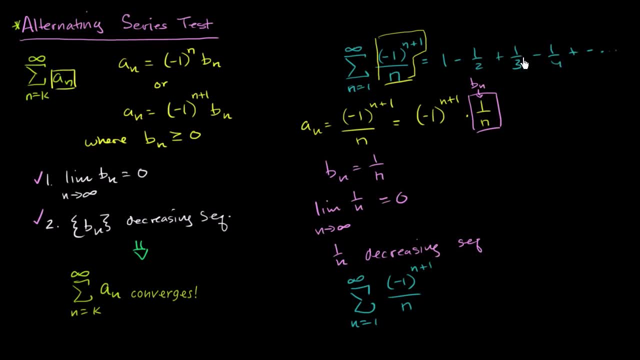 that if all of these were positive, if all of these terms were positive, we just have the harmonic series and that one didn't converge. But this one did. putting these negatives here do the trick And actually we can prove this one over here converges using other techniques. 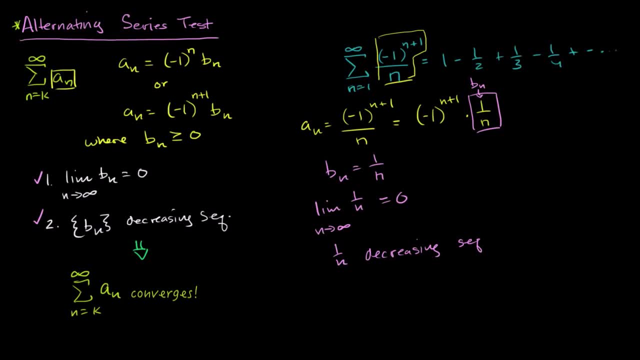 It's a decreasing sequence. Therefore we can say that our original series actually converges. So n equals one to infinity of negative, one to the n, plus one over n. And that's kind of interesting Because we've already seen that if all of these were positive, 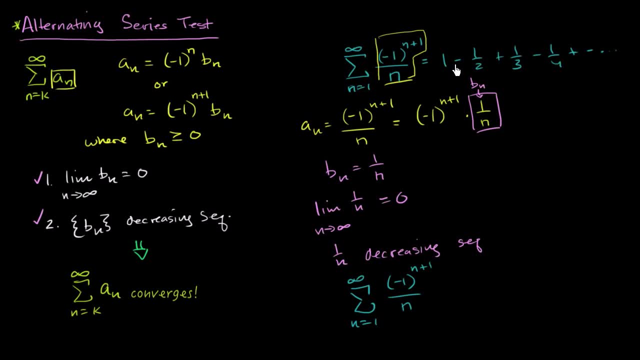 if all of these terms were positive, we just have the harmonic series and that one didn't converge, But this one did. Putting these negatives here do the trick And actually we can prove this one over here converges using other techniques And maybe if we have time. 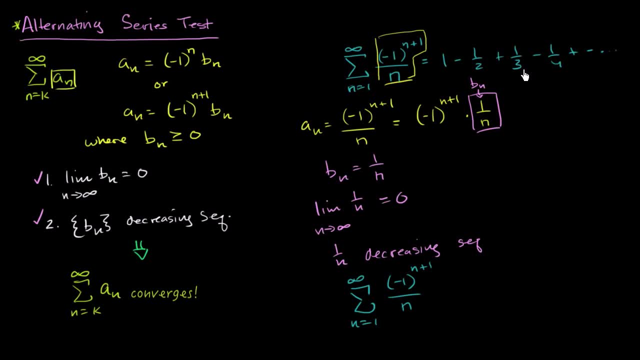 actually in particular the limit comparison test. I'll just throw that out there in case you are curious. So this is a pretty powerful tool. It looks a little bit like that divergence test, but remember, the divergence test is really is only useful if you want to show something diverges. 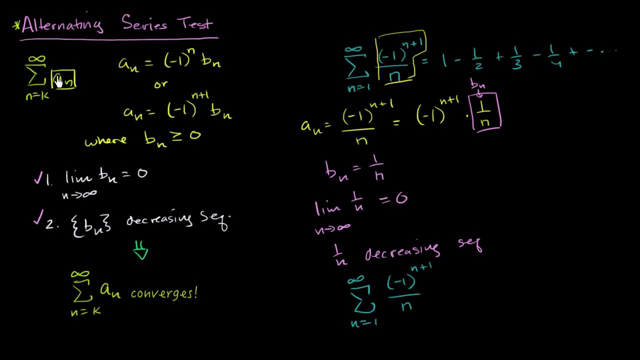 If the limit of your terms do not approach zero, then you say, okay, that thing is going to diverge. This thing is useful because you can actually prove convergence. Now, once again, if something does not pass the alternating series test, that does not necessarily mean that it diverges. 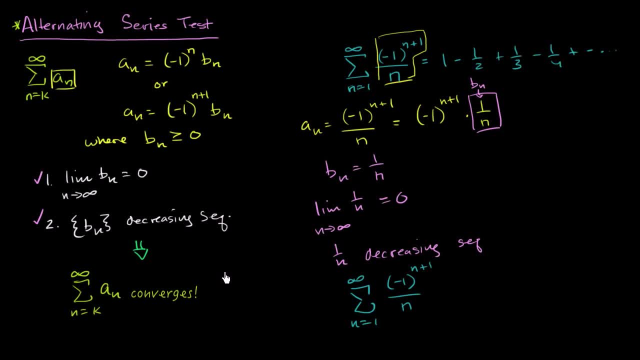 It just means that you couldn't use the alternating series test to prove that it converges. 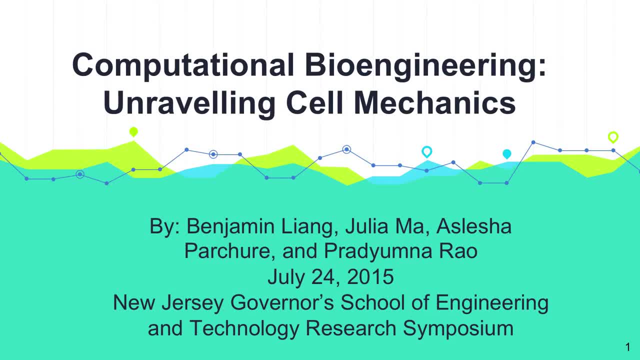 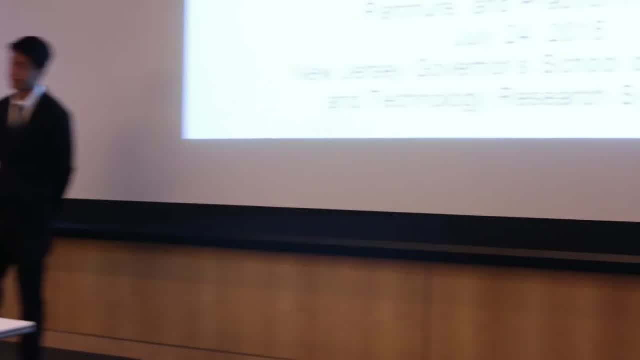 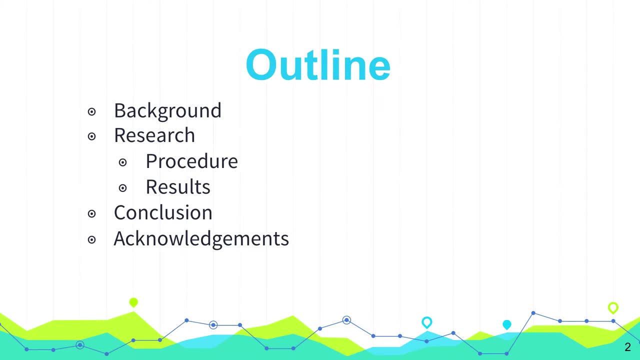 Hello, our research project was Computational Bioengineering, Unwrapping Cell Mechanics and Computers. My name is Ben, I'm Julia, I'm Asleisha And I'm Prad. This is a brief outline of our presentation. We will start with the background information relevant to our project. Then 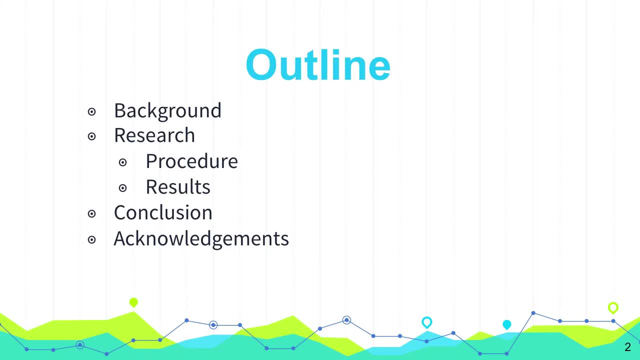 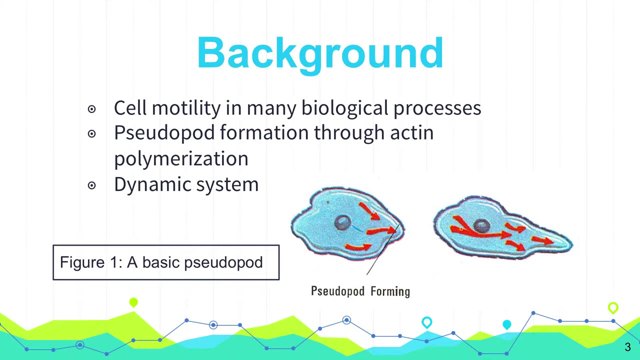 we will talk about our research, which consists of the procedure we did and the results we obtained. Then we will talk about our conclusion from the project. Lastly, we will end with our acknowledgments. Cell motility, or the motion of cells, is a phenomenon that occurs. 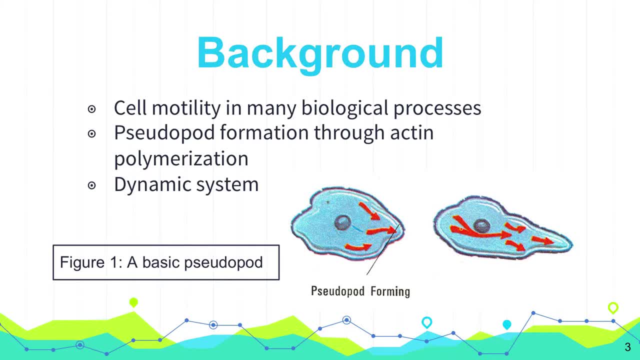 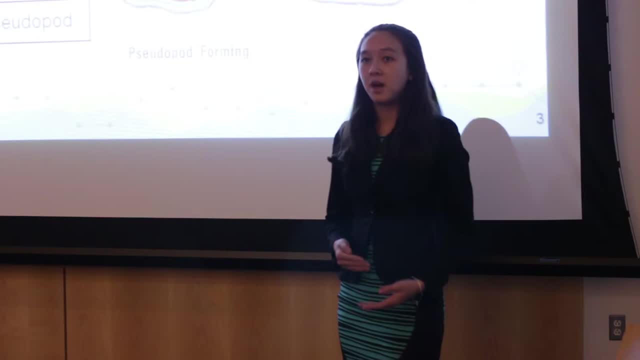 in many biological processes and is present in all living organisms. It is especially helpful in nerve cells, wound healing, immune responses and the metastasis of cancer, which is what causes it to become deadly. Cell motility can occur when pseudopods form within a cell.